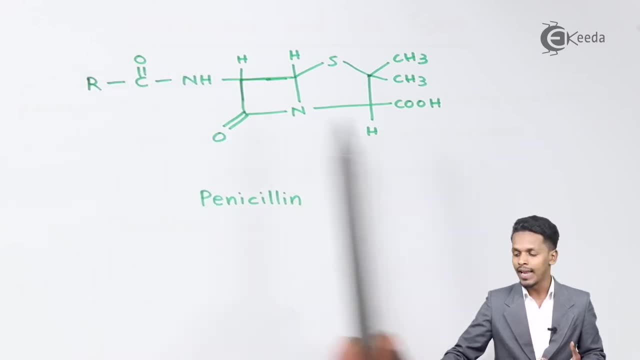 that would be associated to C double bond or NH. that is an amide group and here also we can see that is carboxyl group that is present over here, and these are the two methyl groups and here basically we can see a carbonyl group. So therefore, this is the structure of penicillin and this is the 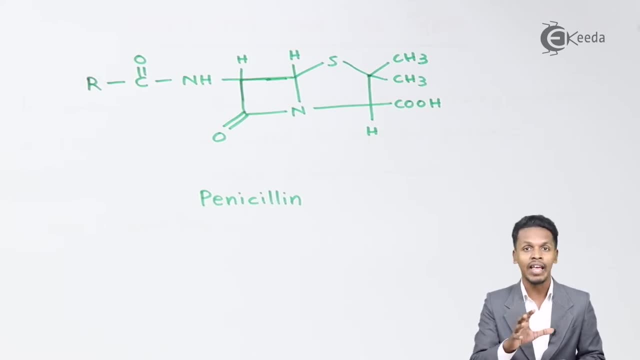 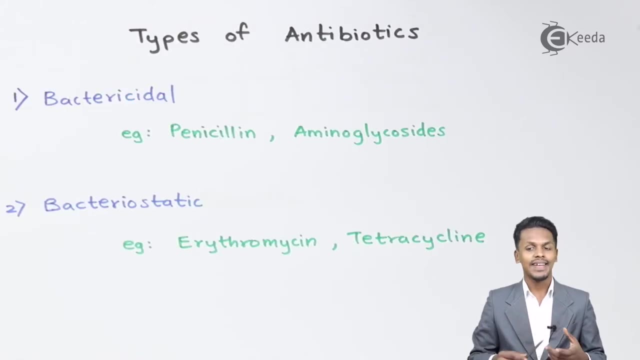 most important structure. that is what we have to do for chemistry in everyday life's chapter. So, talking about the antibiotic, the antibiotics are of different types. So those two different types are, that is, bactericidal and bacteriostatic. So 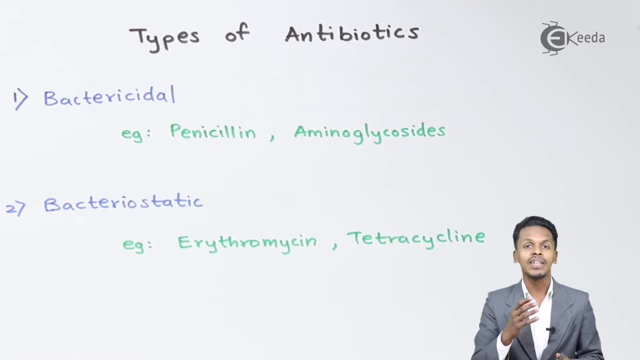 bactericidal is nothing but are those antibiotics which have the tendency to kill the microorganisms and or to kill the bacteria. So in this case, basically example: like penicillin and that is aminoglycoside. So this are basically the bactericidal and talking about the next, that is, 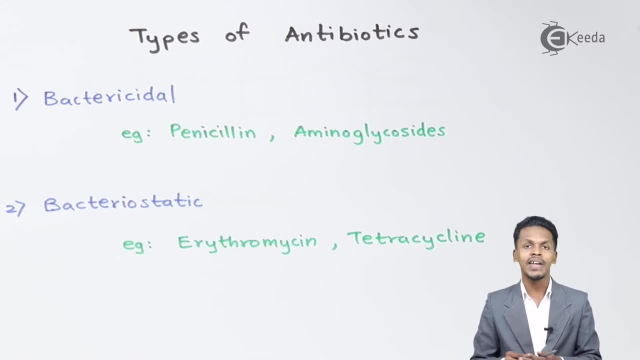 bacteriostatic. So what is bacteriostatic? It is nothing, but it is. it is the antibiotic which stops the growth of the microorganisms, and that's the reason the name is bacteriostatic. So, talking about the examples, that is erythromycin, that is tetracycline, So 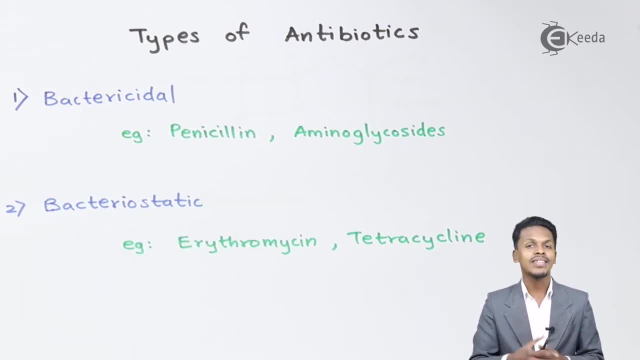 these are the examples of the bacteriostatic. and now let us understand the other classifications of the antibiotic. So antibiotics are also classified depending on the bacteria. So antibiotics are classified by the spectrum of action. So based on that they are basically. 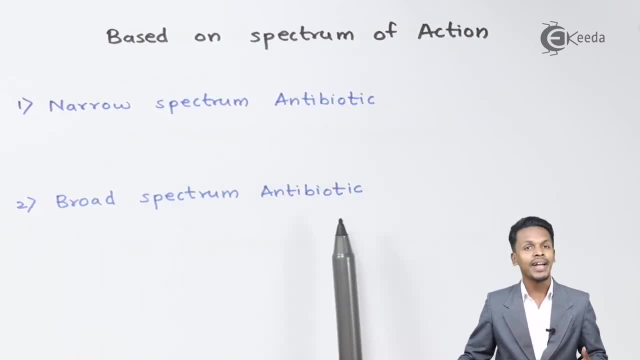 divided into two types, and those types are narrow spectrum antibiotic and broad spectrum antibiotic. So what is narrow spectrum antibiotic? So, those antibiotic which have an effect against either gram-positive or even gram-negative bacteria. those are known as narrow spectrum antibiotic And talking about broad spectrum antibiotic. So therefore, these are the antibiotics which have 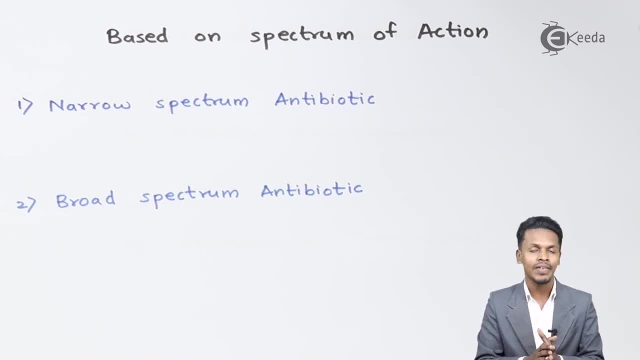 a wide range of action and that can affect both the gram-positive as well as gram-negative bacteria, And those are known as broad spectrum antibiotics. So this was nothing but a small example related to what is actually antibiotic and what are the types of antibiotic, and that's it So.